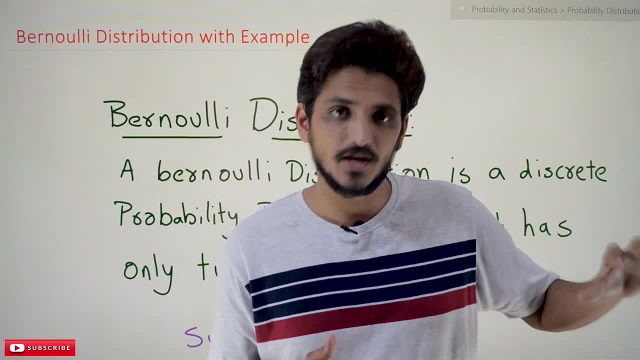 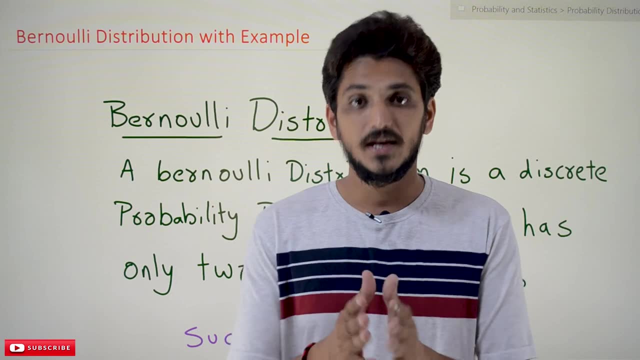 is expected value, what is variance, and all those things were covered in our previous classes. Please watch those classes and come back here. We use all the concepts in this class. The link for the playlist is provided in the description below. Coming to today's class, Bernoulli distribution is: 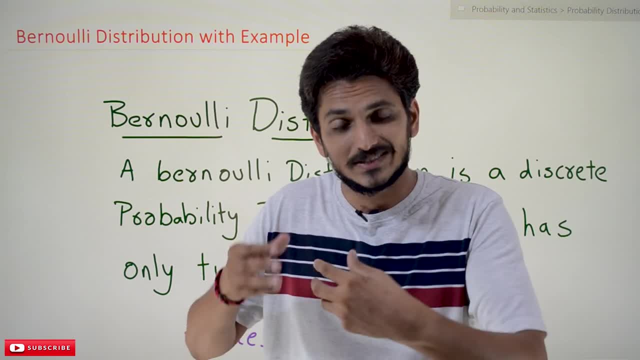 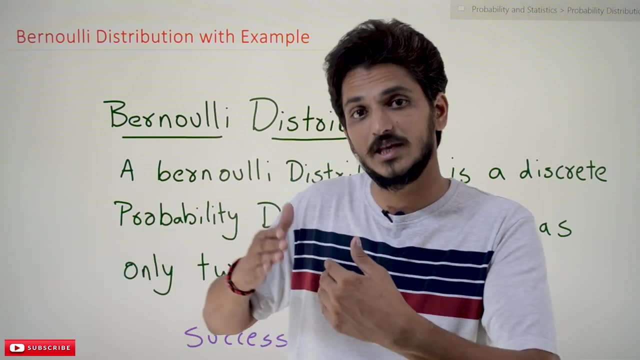 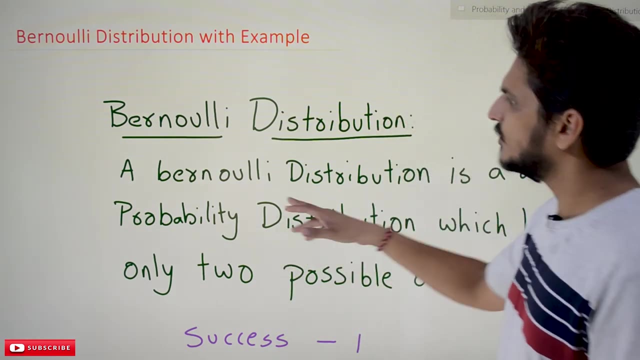 very, very easy to understand. but this Bernoulli distribution is used in our coming classes in binomial and Poisson distribution. Everything is linked to one by one, So please understand it properly so that it helps you a lot in our coming classes. Coming to today's class, Bernoulli- 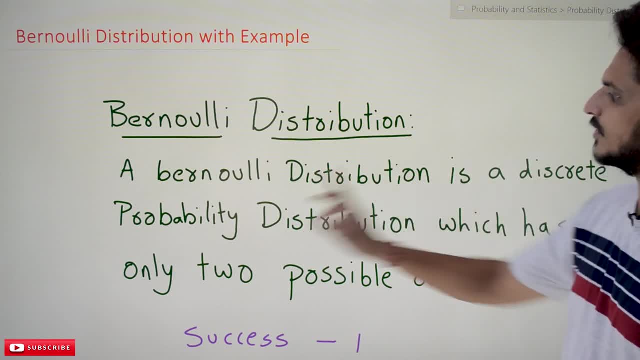 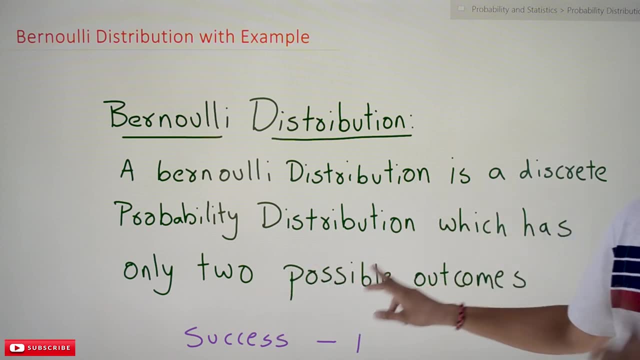 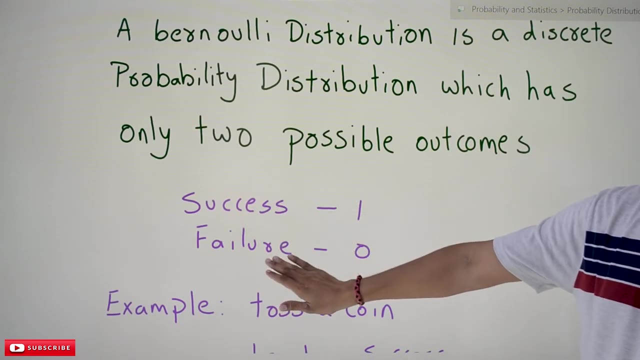 distribution, A Bernoulli distribution, is a discrete probability distribution. It is a discrete probability distribution which has only two possible outcomes. Those outcomes, one we call it as success and the second one we call it as failure. Success is given a variable value: 1 and failure. 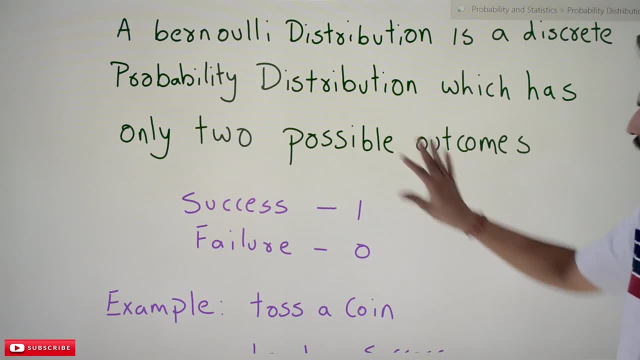 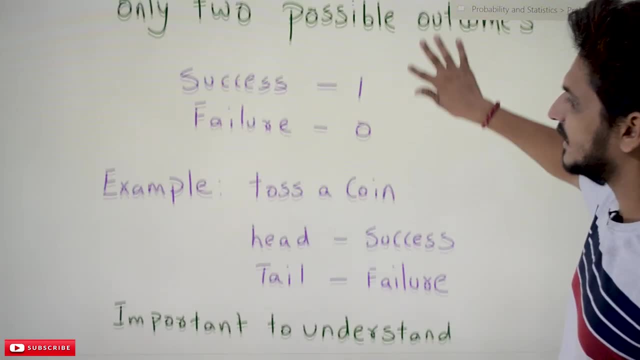 is given a value of 0. If you are having only two possible outcomes, then we call it as Bernoulli distribution. With example you will get clarity. Let's take an example. toss a coin. We are having only two possible outcomes. 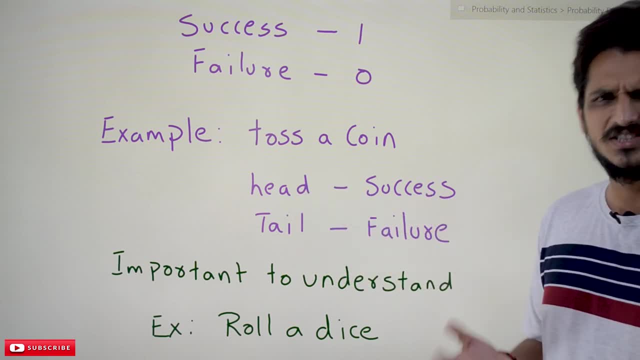 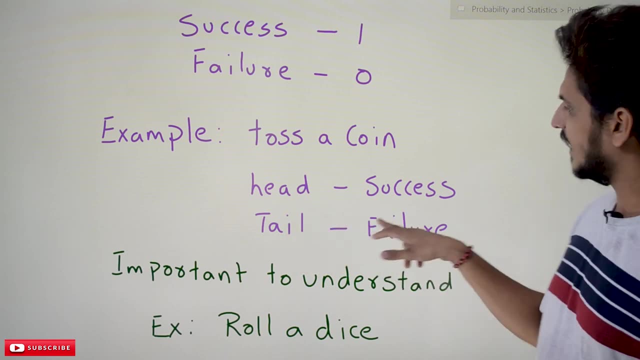 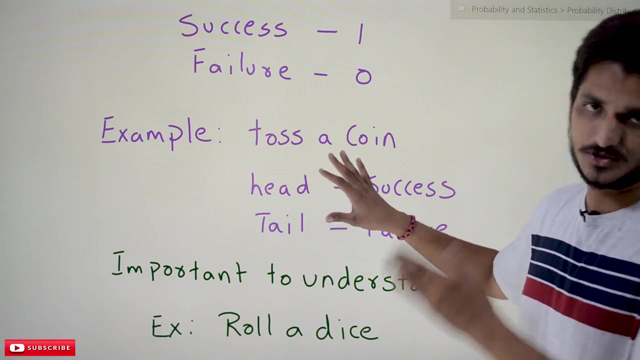 head, tail. Head is considered as success. Is it compulsory to consider head as a success? No, In our experiment, we are considering it as head as success. Tail is tail as failure. This is this, this tossing a coin. you can postulate it into Bernoulli distribution. 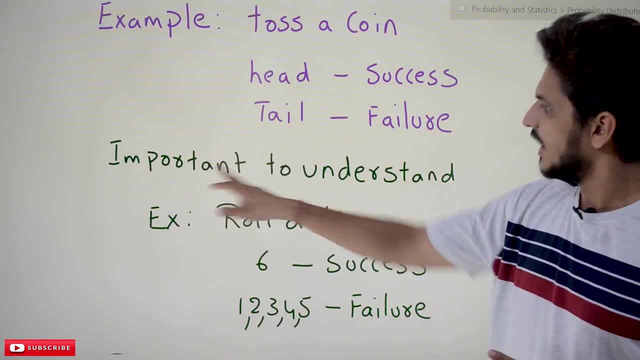 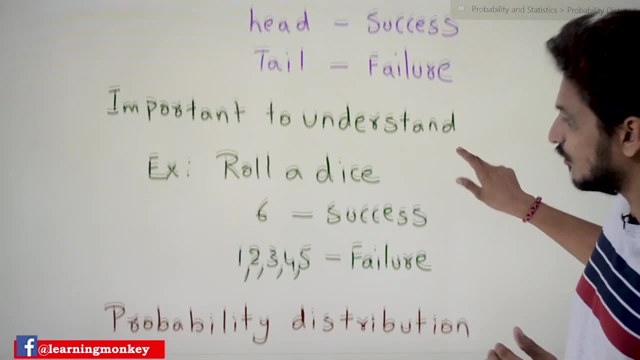 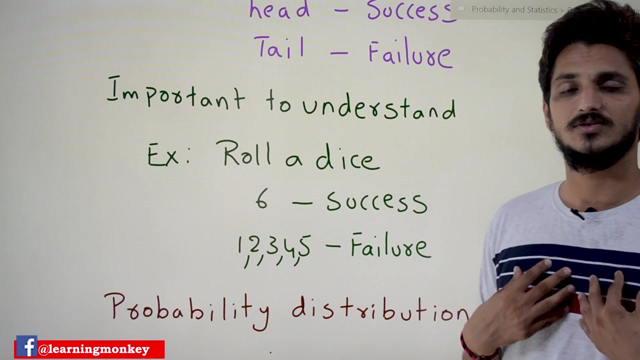 Similarly, one important point you have to understand from the definition. important to understand is roll a dice. Yes, it is also a Bernoulli distribution. How, how it's happening like a Bernoulli distribution. Let's consider it as a 6 is considered a success When you 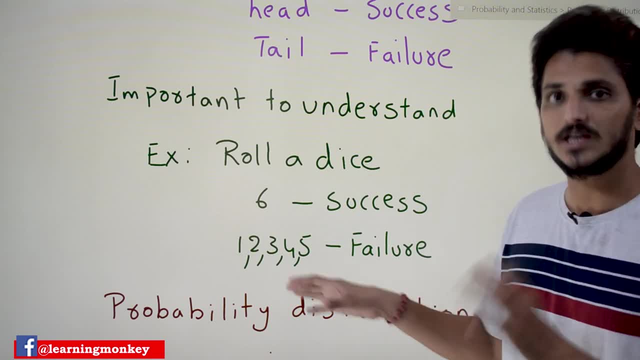 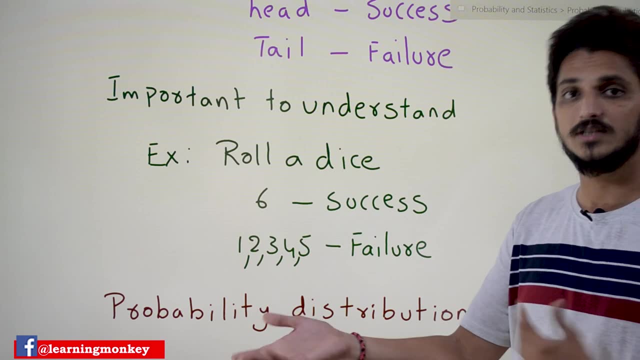 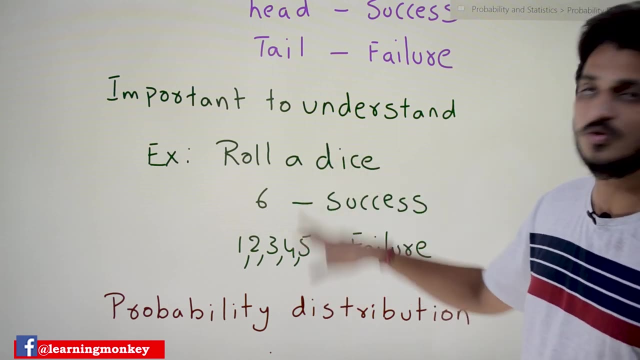 roll a dice. in our experiment we are considering 6 as success, remaining as failure. So we are having only two possible outcomes When you roll a dice. it may be success, it may be failure. This also considered as a Bernoulli distribution. This is the point you have to understand. 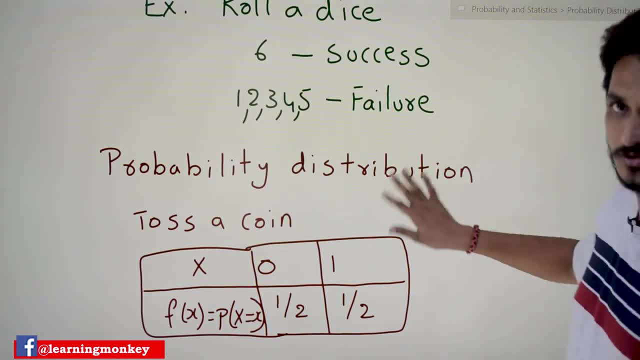 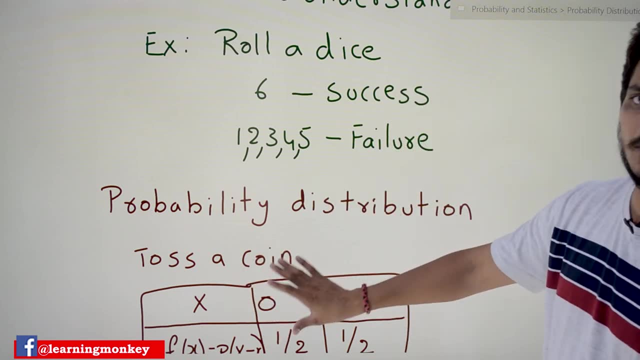 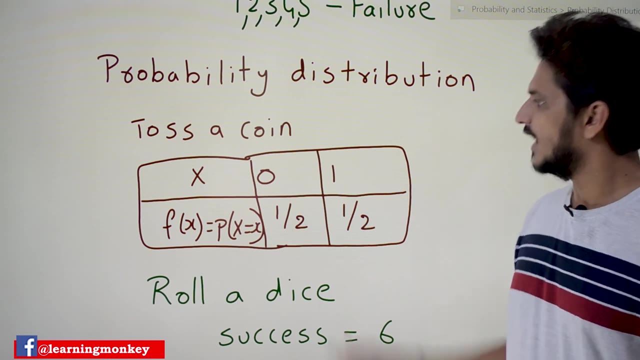 Now coming to our probability distribution. So for the same Bernoulli, Bernoulli probability distribution. we are showing the probability tables, distribution table, so that you will have better understanding of Bernoulli distribution. Tossing a coin: what's our random variable? Xs: Either 0 or 1.. 0 means failure, 1 means 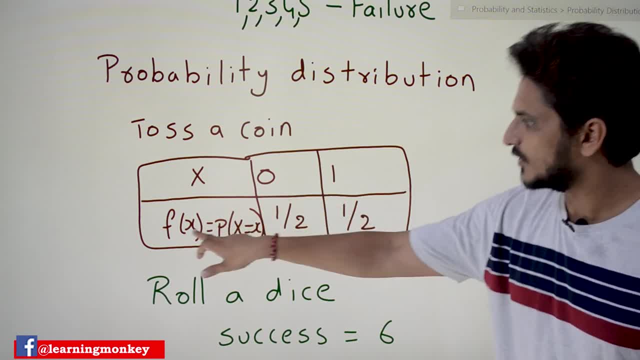 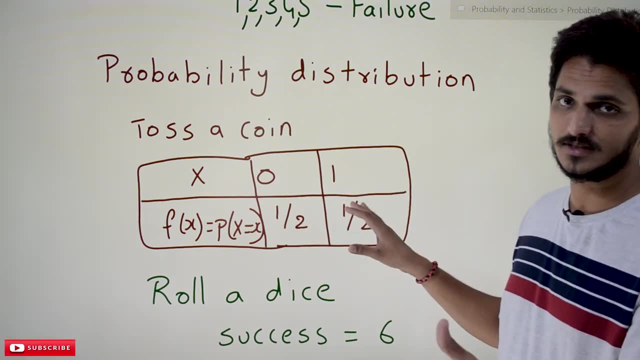 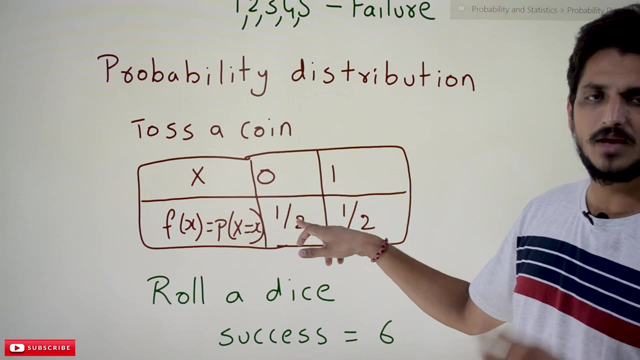 success. so what is the probability f of x? probability of x is: this is what probability distribution table means. this we already discussed in our previous classes. probability distribution table for Bernoulli distribution is like this: for 0- tossing a coin, what is the probability 1 by 2? for 1, what 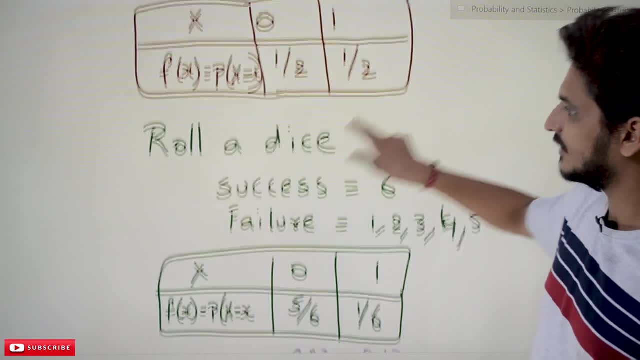 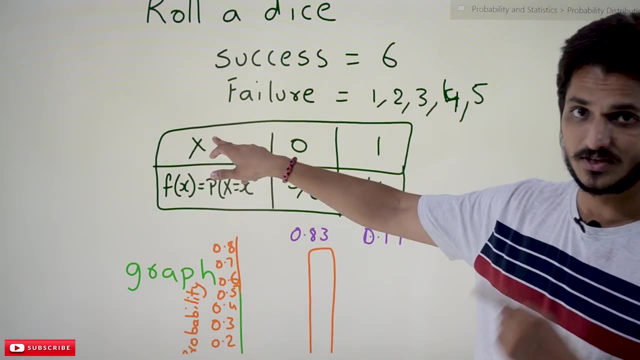 is the probability: 1 by 2. similarly, or second rolling a dice, success is considered as 6, failure is considered as 1, 2, 3, 4, 5. so x is equal to x. means random variable. x is 0 or 1, f of x is given. 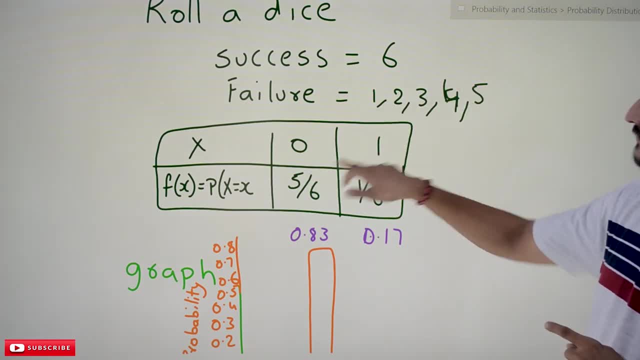 as a 0. how many possibilities are there? 5 possibilities. that's why 5 by 6 success. how many possibilities? one possibilities, that is 1 by 6. 5 by 6 means, on an average it is a. it is not the exact value: 0.83, something will come approximately 0.83. 1 by 6 means 0.17, like this: 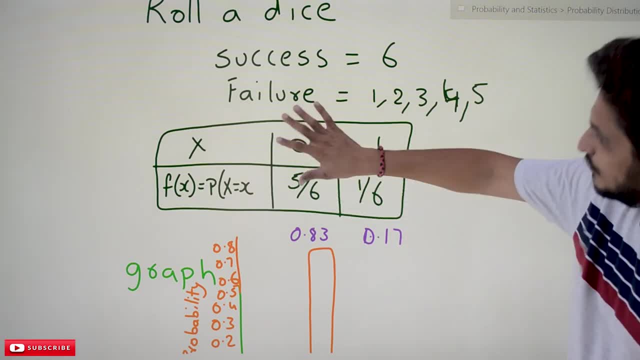 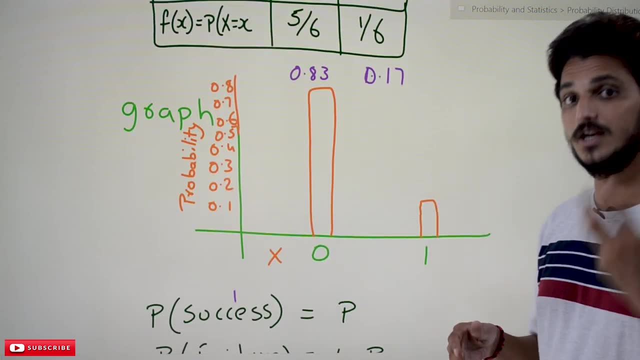 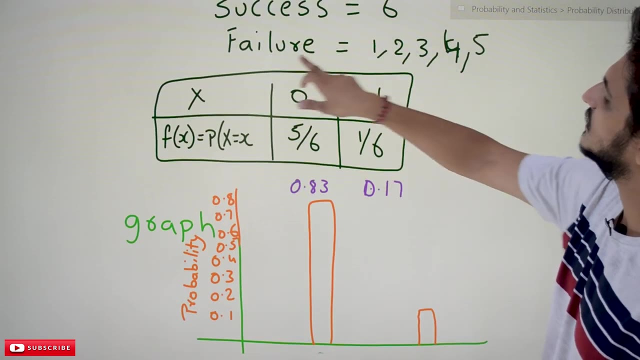 so how we graph it. graph the Bernoulli distribution. that is also very important to understand. graphical intuition will have help you a lot in understanding the concepts. so if you plot the Bernoulli distribution for rolling a dice, success is equal to 6, failure is equal to 1, 2, 3, 4, 5. 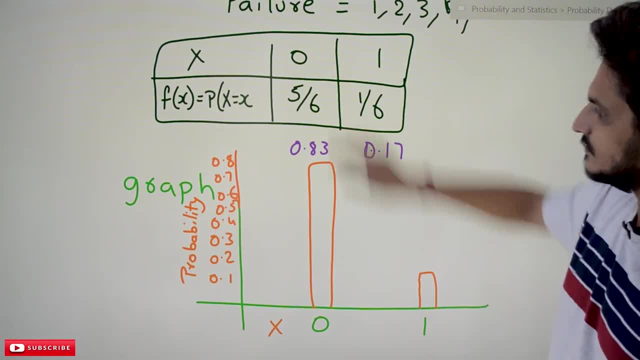 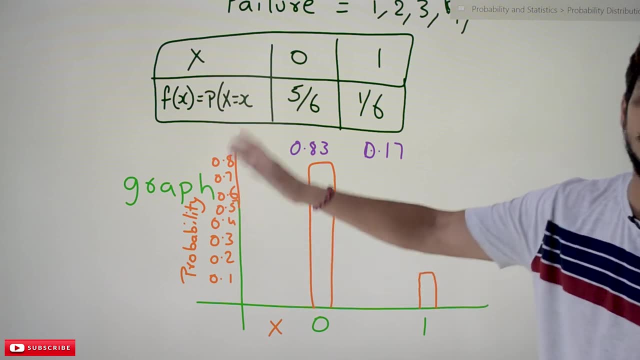 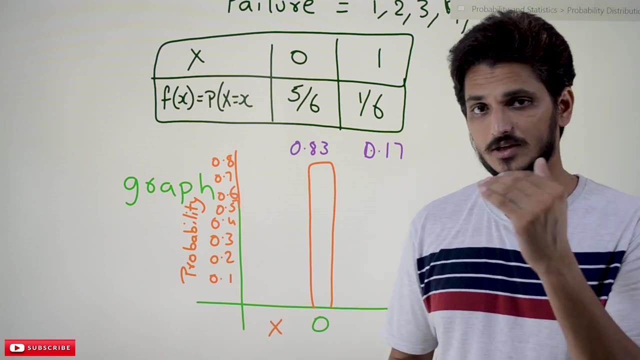 so the probability distribution is like this. so this: we are plotting it. on the x axis, we are taking a random variable, 0 and 1. on the y axis, we are taking the probability values. so 0.1, 0.2, 0.3, so on, what's the maximum probability value? you are having a 1. so what's on the y axis? 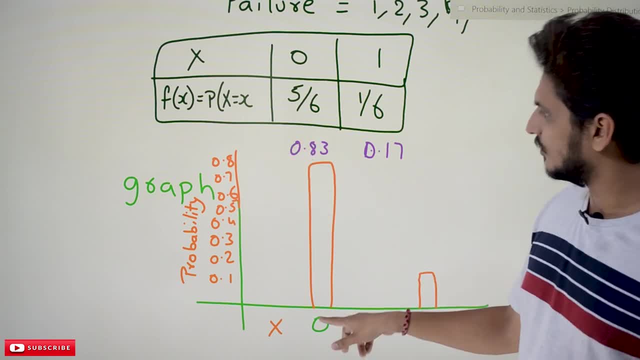 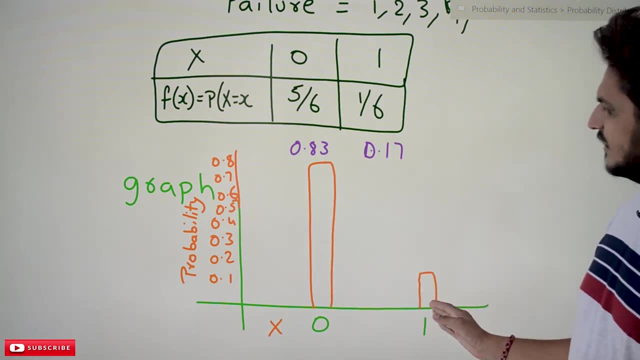 what's the maximum value? will have 1, so 0. what is the probability? 0.83, something. that's why our distribution is like this: 1. what is the probability value? you are having 0.17, so that's why the graph is like this. this is how we will. we will graph the probability distribution: discrete probability. 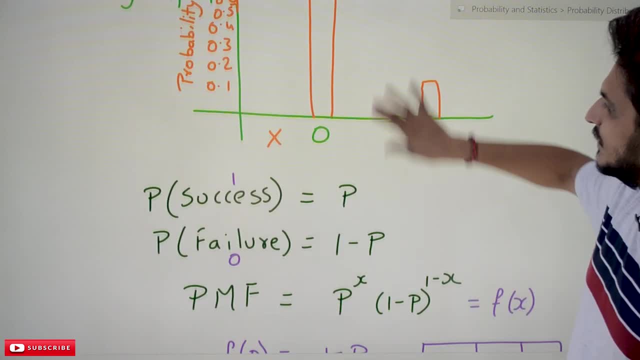 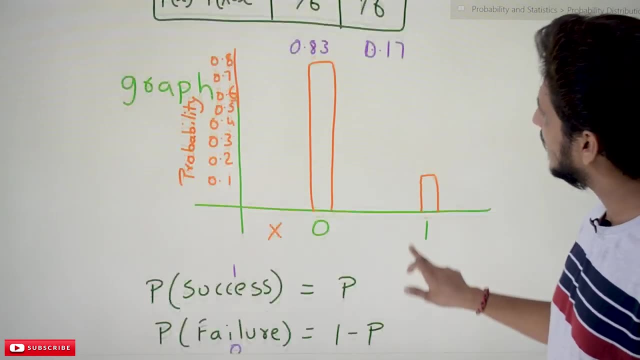 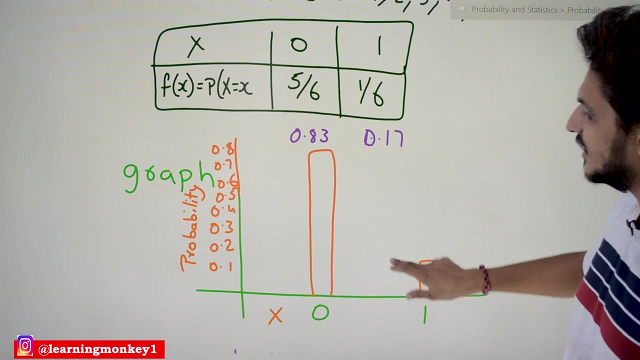 distribution. okay now, coming to that, it probability of success means we consider it as success is considered as 1. the same experiment in the same experiment. so what is the probability of success? 1 by six is considered as p. if you consider 1 by 6 SP, what is probability of failure? and I'm mining all. 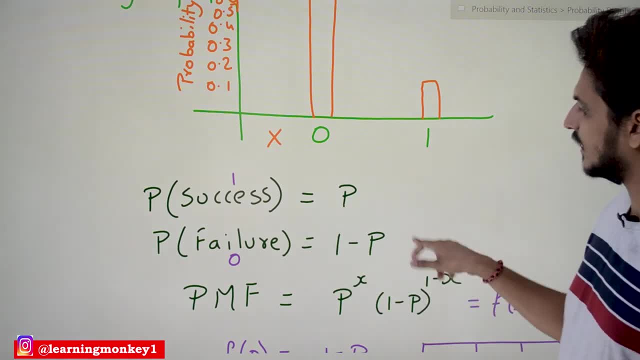 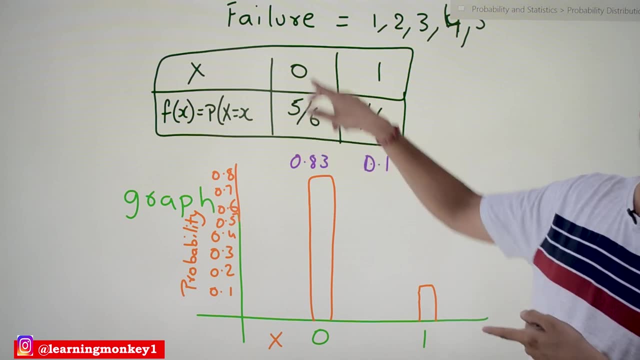 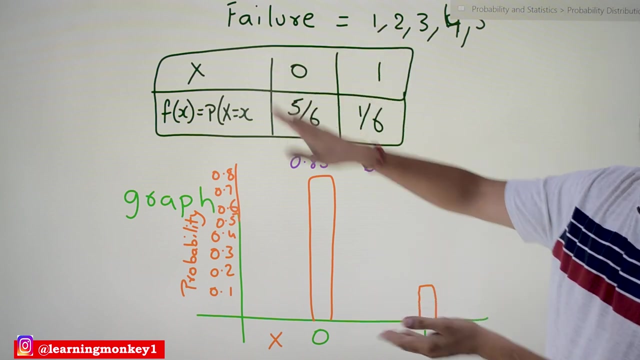 we considered at test failure. so that which is 1 minus P, 1 by six is there is our success. 1 p means 5 by 6 is our failure, because bernoulli distribution having only two variables if it is not this other one. so that's why probability of success one is given as a p probability of failure. 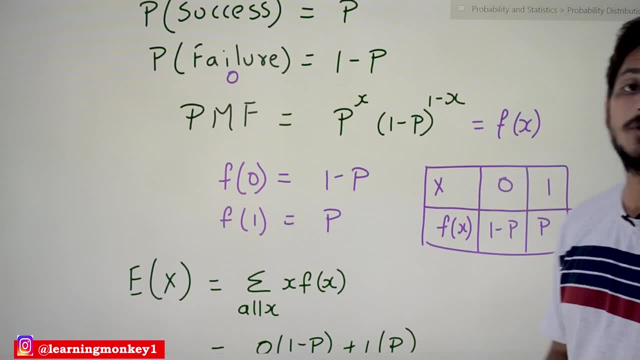 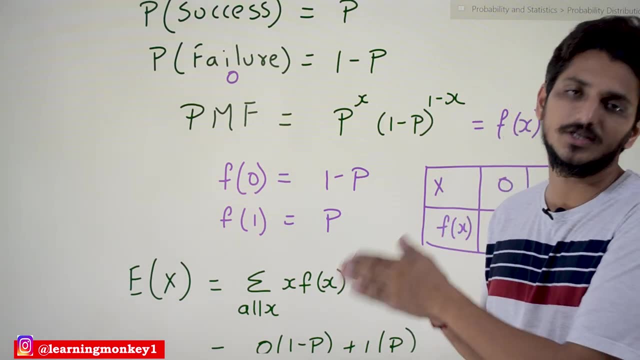 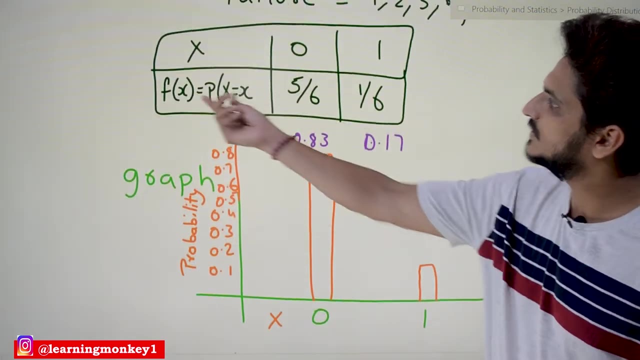 is given as 1 minus p. now coming to the probability mass function. so what is the probability mass function for bernoulli distribution? so don't get confused. in our previous classes we clearly discussed this f of x, which is giving the probability value that we for discrete probability. 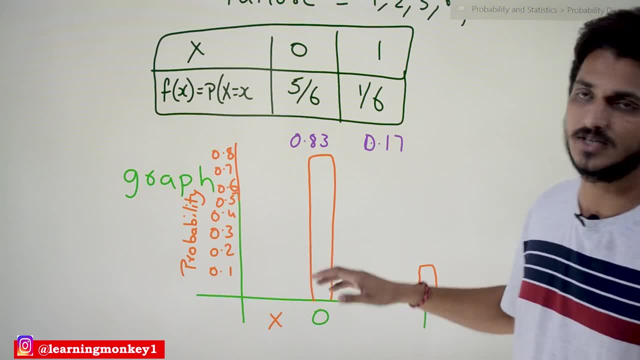 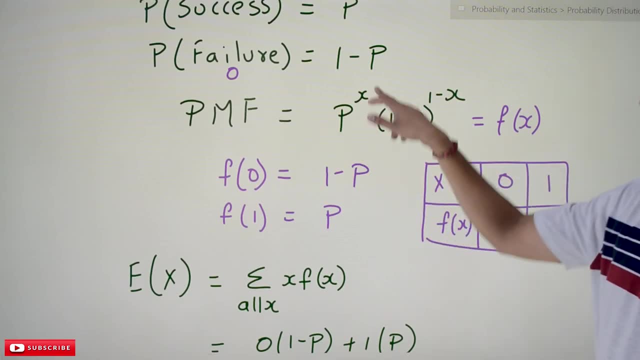 distributions. we call it as probability mass function means we are we are finding the f of x for bernoulli distribution. so probability mass function is equal to p power x multiplied by 1 minus p power, 1 minus x. that is equal to f of x, means probability mass function, which is we call. 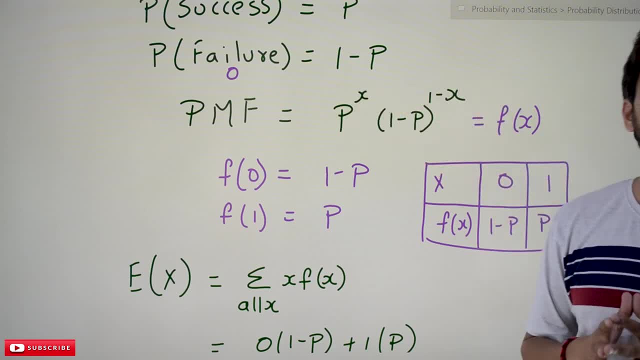 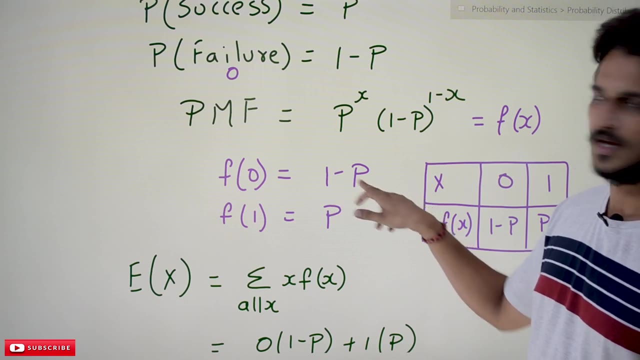 it as f of x. this is our bernoulli distribution, probability mass function. why? why it is probability mass function for bernoulli distribution. that is the point you have to understand. if you substitute f of f of 0 means 0 in this, we'll get 1 minus p if you. 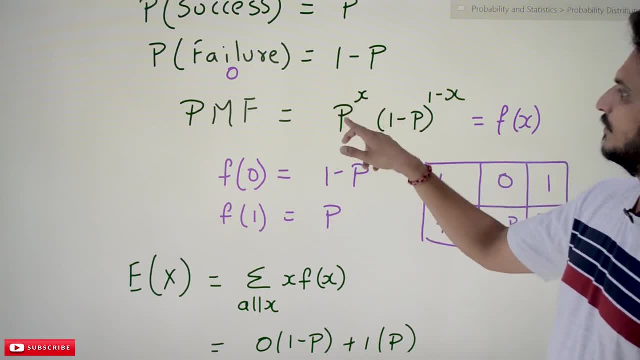 substitute 1- 1 in this equation, we'll get p. p power 0 means anything. power 0: 1, 1 minus p. power 1 minus 0 means 1, 1 minus p. so f of 0. if you substitute 0 in this equation, we are getting 1. 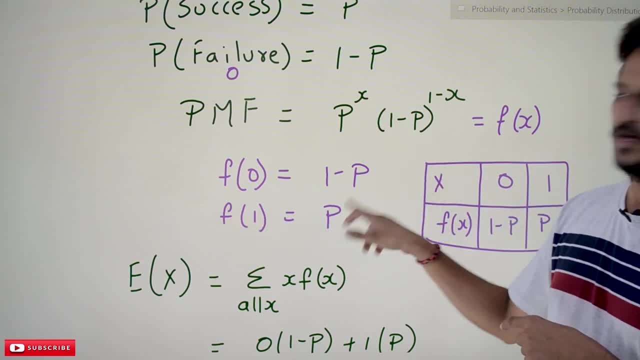 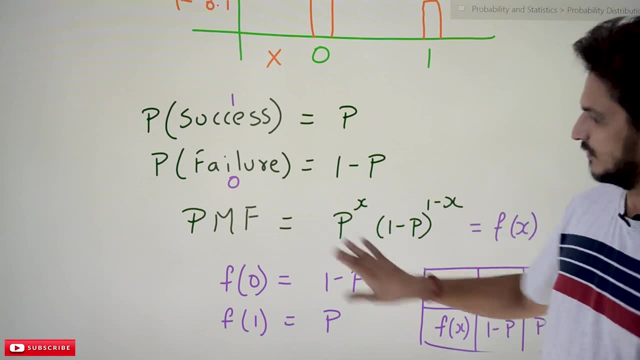 minus p. if you substitute 1 in this equation, we are getting 1 minus p. if you substitute 1 in this equation, we are getting p. this is what our bernoulli probability of success is p. probability of failure is 1 minus p. probability of failure is 0. so if you substitute 0, 1 minus p, if you 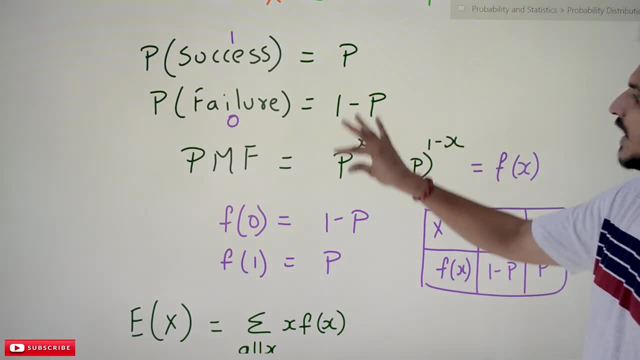 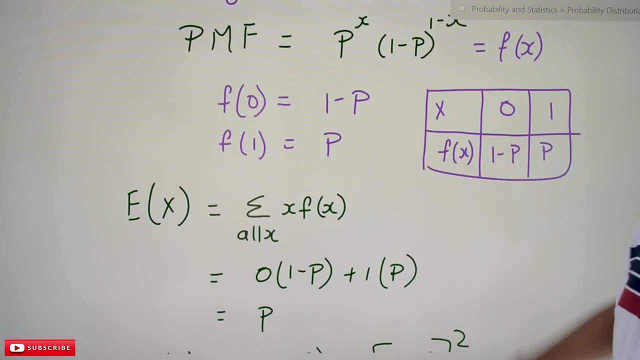 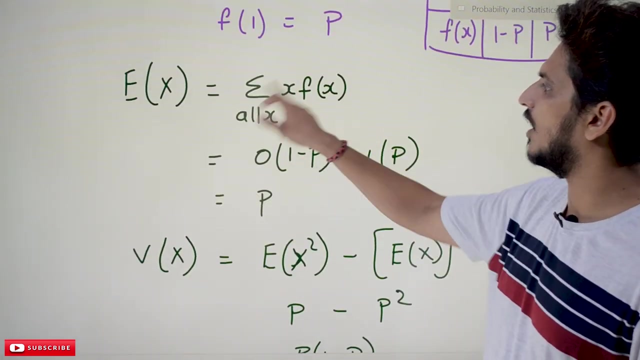 substitute 1, p. so this is the probability mass function for bernoulli distribution. if you know the probability mass function, we can find the expected value. we can find the variance value. also, how we find the expected value. expected of x is equal to sigma all x, x, f. 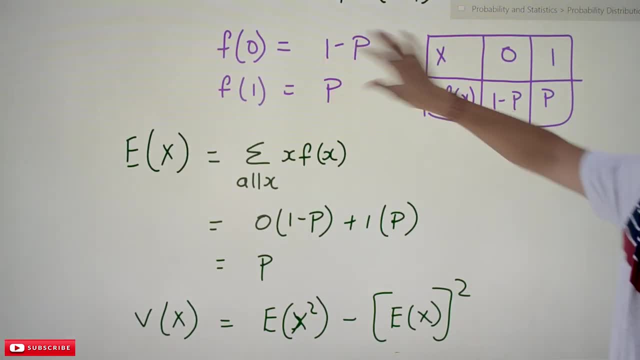 of x. so if you plot the bernoulli distribution x, 0, 1, 0 means failure, we will get f of x. value is 1 minus p, 1 means p, so x. f of x means 0 multiplied by 1 minus p. it's 0 plus 1 multiplied. 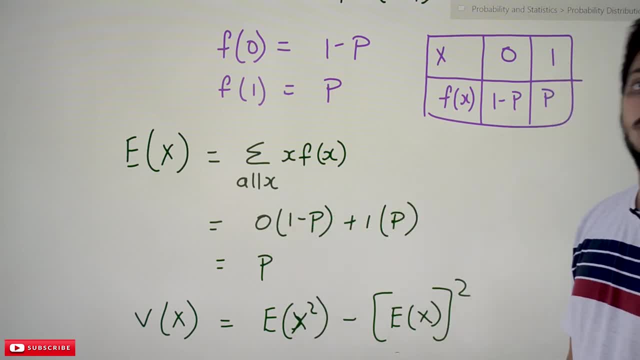 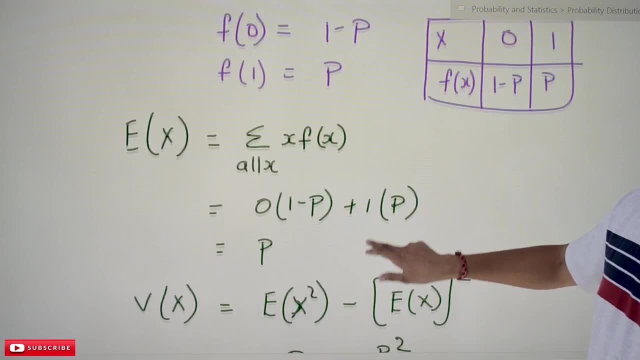 by p. so expected of x is p. so what is expected of x? already discussed what's that value means. so p is the expected value of bernoulli distribution. similarly, if you plot the bernoulli distribution, x, 0, 1, 0, x, f of x value is 1 minus p. so x, f of x. 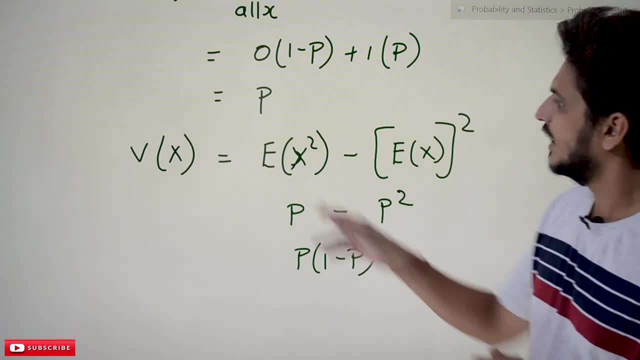 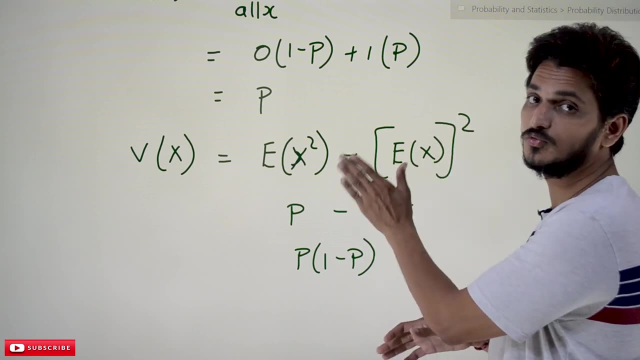 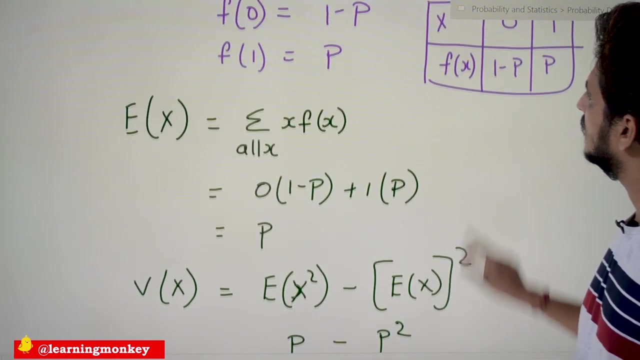 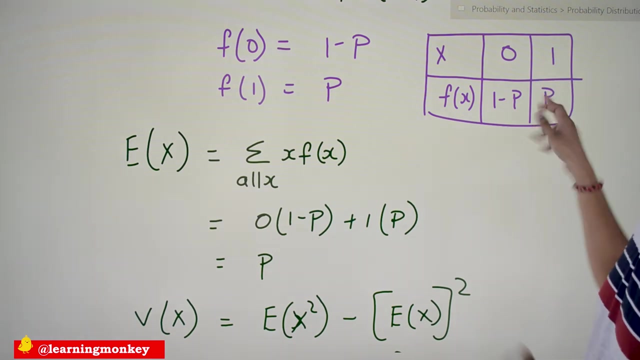 if you want to find the variance of the bernoulli distribution expected of x square minus expected of x whole square. this is what the equation for variance to find the to find the variance for discrete probability distributions expected of x square means. in this equation, if you place x square f of x, x square means 1 square multiplied by p, 0 square multiplied. 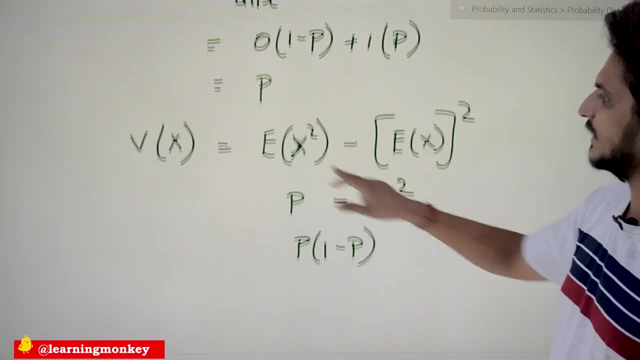 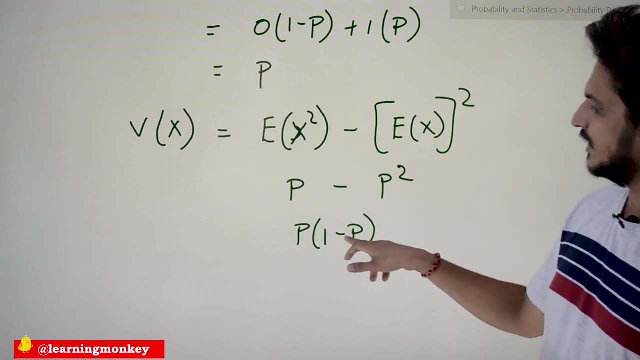 by 1 minus p, which is equal to p. So the variance of x square is p minus expected of x whole square is equal to p square, that is, p multiplied by 1 minus p. we are not concentrating what is expected of x square and how to find. 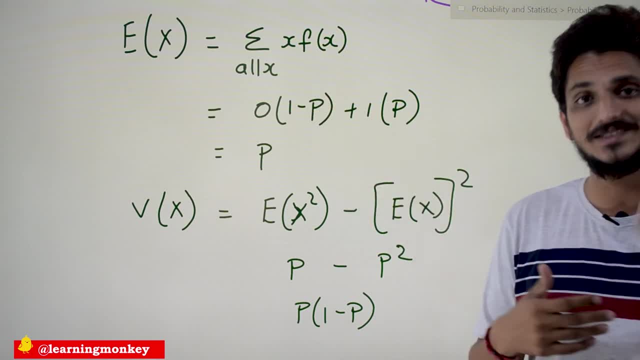 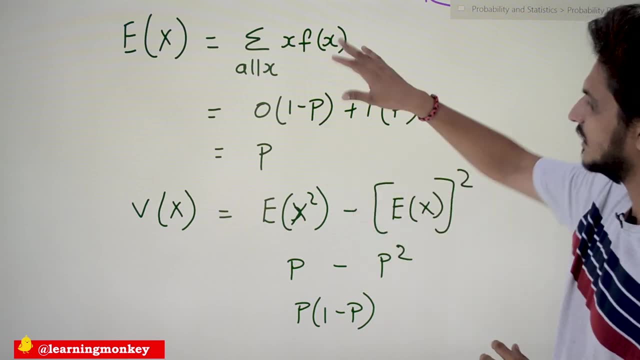 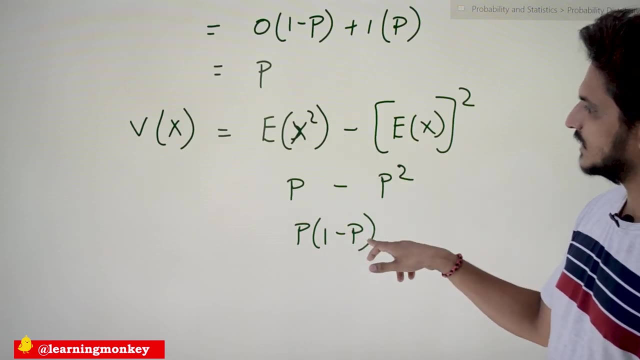 the expected of x- x square, because we made some examples in our previous classes how to find this variance and expected value. hoping that that's why we are not concentrating on the substitution and finding the equation. so this is what the p multiplied by 1 minus p is the variance of bernoulli distribution. hope you understand this bernoulli distribution. 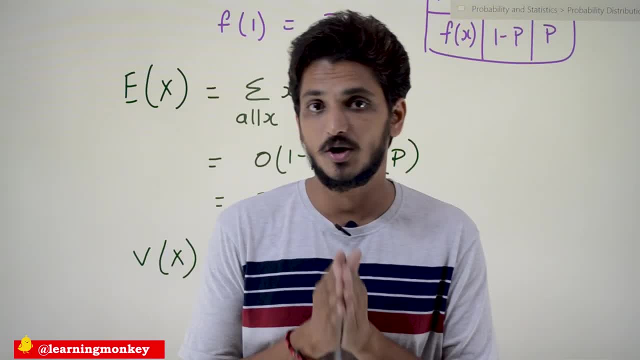 if you have any questions regarding the concept, please post your questions in the comment section below. thanks for watching. if you haven't subscribed to our channel, please subscribe to our channel and press bell icon for the latest updates. thank you.